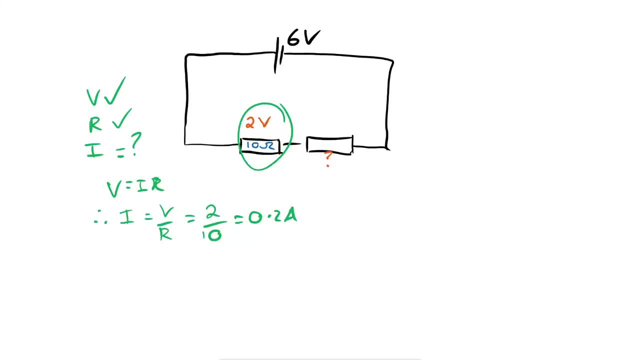 And that gives us 0.2 amps. Now, that's fairly easy, But then it's the rules that people forget. What do we know is true for this circuit? It is a series circuit, And so we say that if that's the 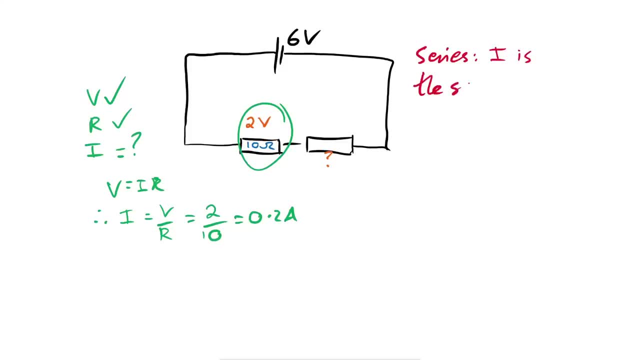 case current, is the same everywhere. So can you see, we found out something about the first component And now we can say that's also true for the second component. here There is one more thing we can say is true for a series circuit, We can say that's also true for the second component. 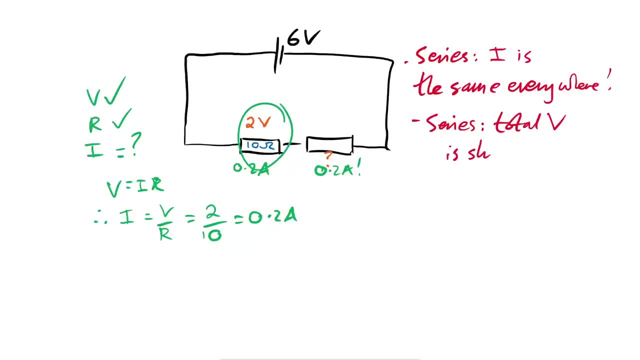 And that is that total V, total voltage, is shared. So therefore, if I know I have six volts available altogether, but two volts is being used to play the first resistor, then that must mean that there's four volts available for the second resistor there. So I now have V, I have I for this. 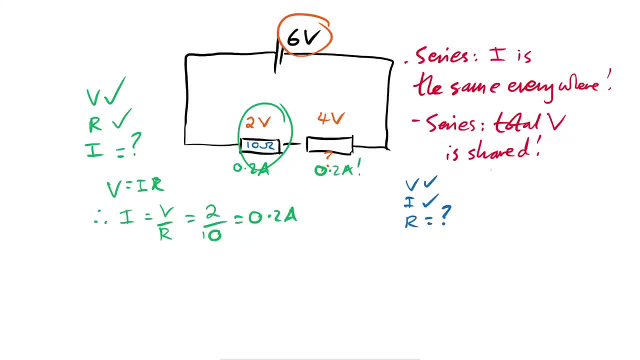 second resistor. What can I find out? I can find out the resistance Rearrange Ohm's law. again, R is equal to V over I in this case, So that's equal to four divided by 0.2. And that gives us 20 ohms. Now, you might well have been able to predict that. 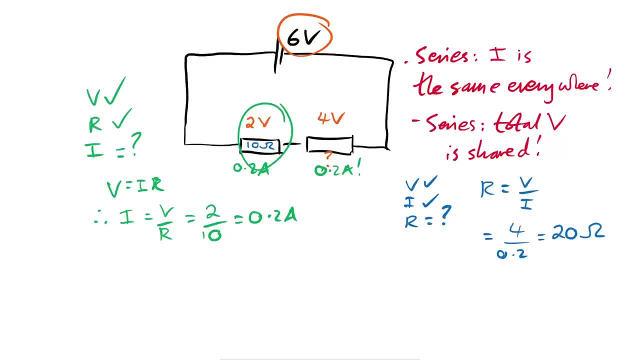 that was going to be the case just looking at the numbers, But it's not always nice numbers like that, And so these rules are super important. Knowing these rules will allow you to say: I found out something for one component. I can therefore use that for another component. In this case, 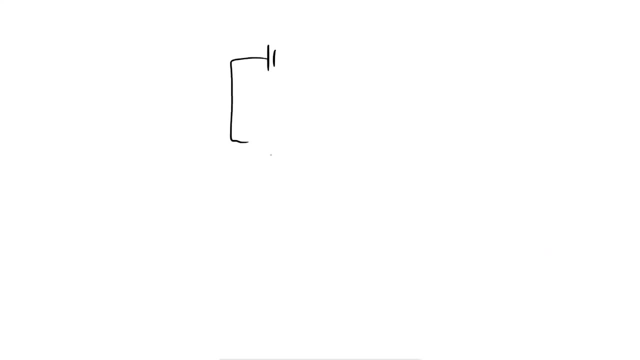 it was the current that was the same for both. Let's look at another circuit. Of course you can probably see that I'm going to be drawing a parallel circuit here. Let's say the total voltage is 10 volts And I know the total current going through the circuit. 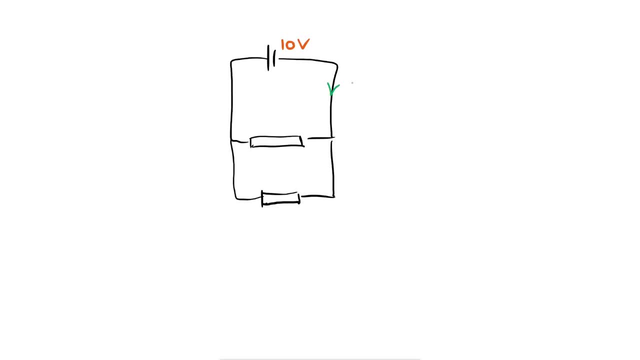 go through the battery, through the cell, they might say as well, is 0.5 amps. I can tell you that this resistor here is 50 ohms. I can tell you that this resistor here is 30 ohms. So it 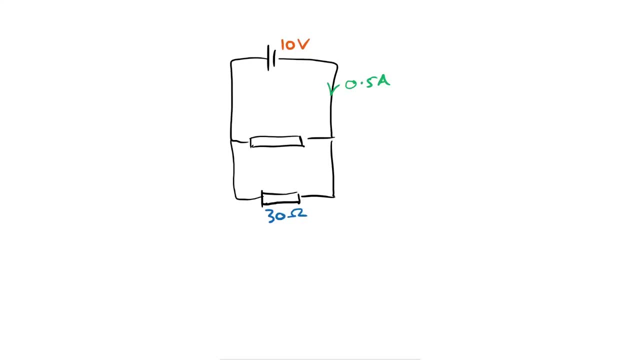 looks like we haven't really been given that much information here, But there's still some things that we can infer. Let's have a look. We know this is a parallel circuit. So if that's the case, we know that, we know that V is the same for all branches- Then if we have 10 volts available, 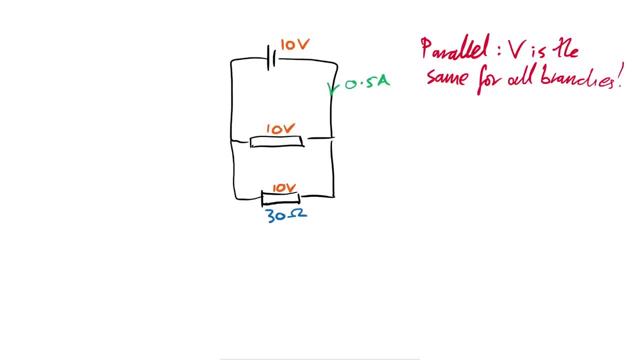 altogether. that means we must have 10 volts across here and 10 volts across this resistor too Cool, Now we're getting somewhere. Let's look at the bottom resistor. We know two things: 10 volts and 30 ohms. We can, of course, find out the current. The current is going to be equal to. 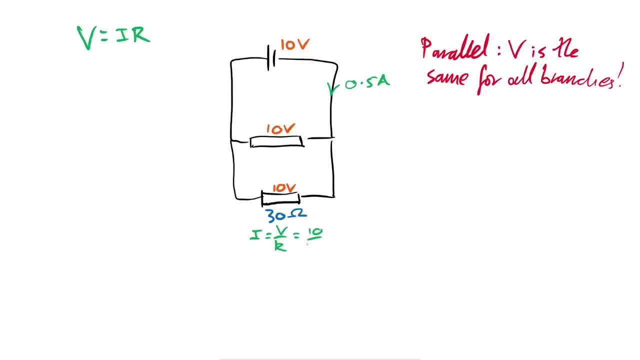 V divided by R, rearranging ohms lower again. So that's equal to 10 divided by 30.. And that gives me well, let's just say 0.33 amps. So that gives me. well, let's just say 0.33 amps. 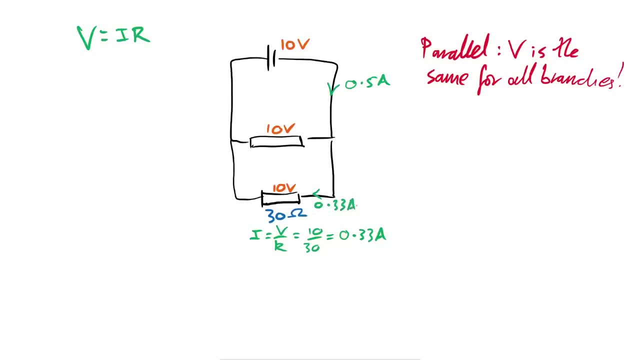 So now I know that there's a current of 0.33 amps going through the bottom branch, But if I know that I have the total current of the circuit of 0.5 amps, well, Kirchhoff's first law if you want to know the name of the law that we use. but 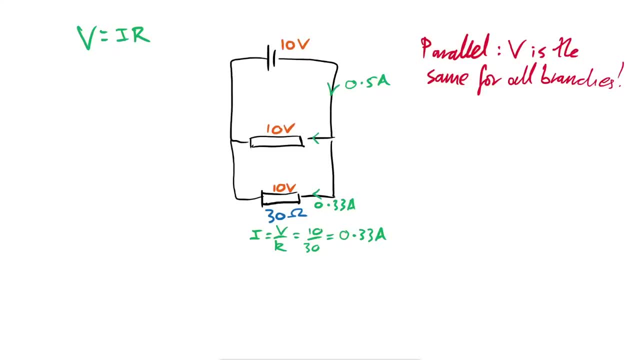 well, you should know that current just doesn't disappear once it goes through branches. If there's 0.5 amps altogether, but 0.33 is going down the bottom branch, that means that one take away the other, This should be 0.17 amps going through this top branch. here Now I have 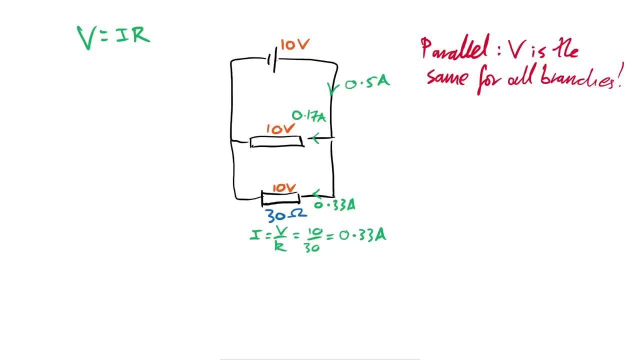 to realize that technically, I've drawn my cell the wrong way around, but we're not too fussed about that. There we go. Current always goes from the long end to the short end, That's positive to negative, Not that it matters too much when we're doing calculations. Therefore, I now know. 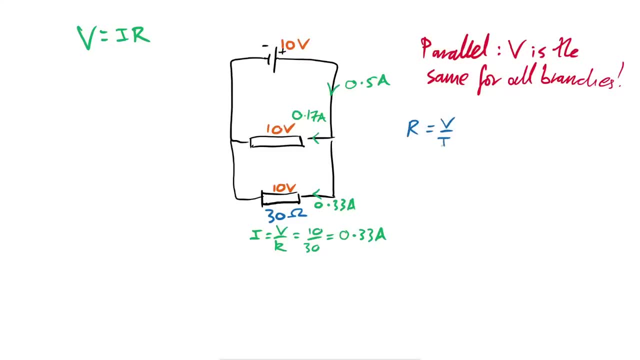 two things about this top resistor here I can do. resistance is equal to V divided by I, so that's 10 divided by 0.17, and that gives me 59 ohms. So there we go again. it was all thanks to this rule. 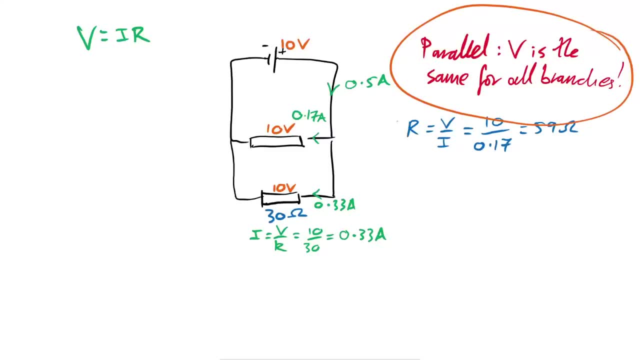 here. Parallel V is the same for all branches, And I can also do this here. I can do that. here There's 0. Меня. Then, of course, we use the other rule as well. Current is always conserved at junctions. 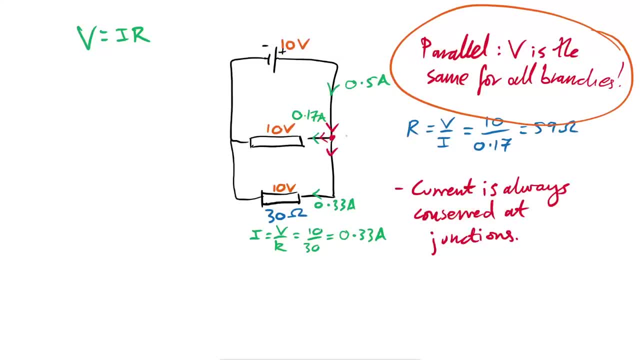 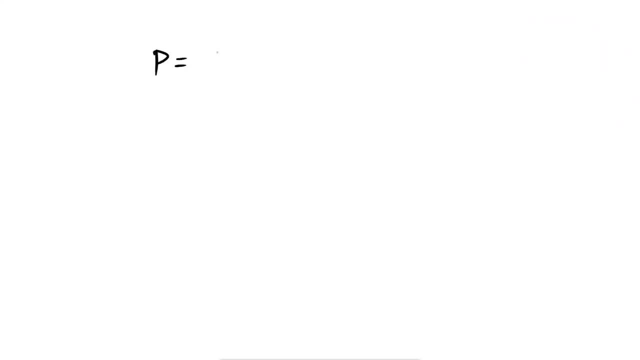 In other words, whatever current goes into a junction here we have to have the same amount coming out altogether. Of course you might have to use power instead. Maybe you're given the power dissipated in watts for a resistor, and that's equal to IV. 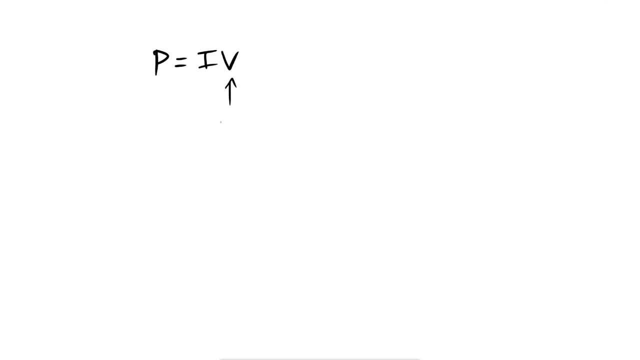 But we can replace INV with Ohm's law. We saw that Ohm's law says that V is equal to IR. So if you replace V with IR, we end up with: well, I times, I times R, so I squared R. 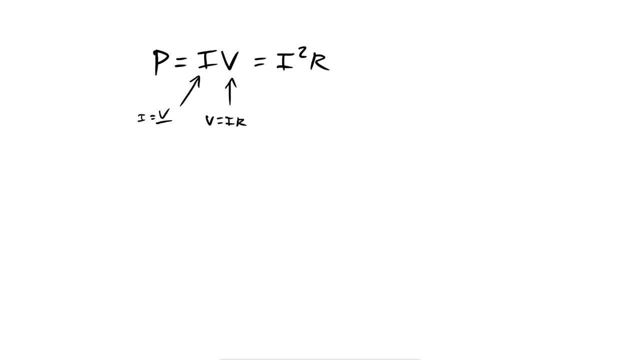 We can also replace I with V over R, So we end up with V squared over R. So again, you just have to know two of these things in order to find out the third: If you know INV, you know P. If you know INR, you can calculate P. 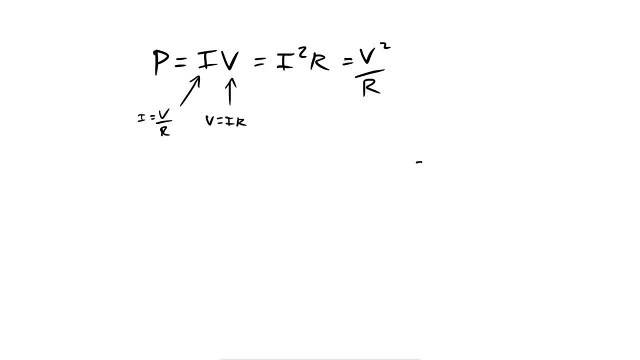 If you know V and R, you can also calculate P. An example of this would be transformers, where we have a primary coil and then a secondary coil. This looks like a step-down transformer, doesn't it? You might have something that says: 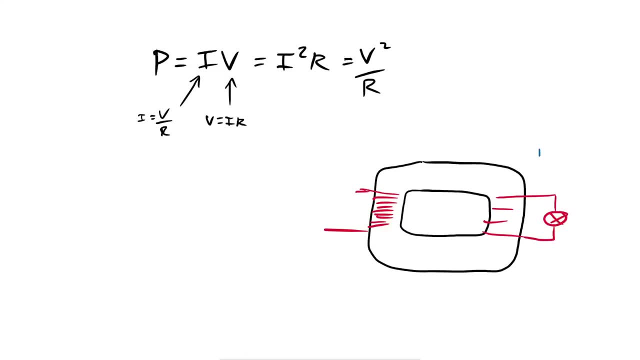 hey, here's a bulb on the secondary coil here and its power is equal to 20 watts And the current going through it is. I'm calling it I2 because this is a secondary coil, This is the primary coil, so one and two. 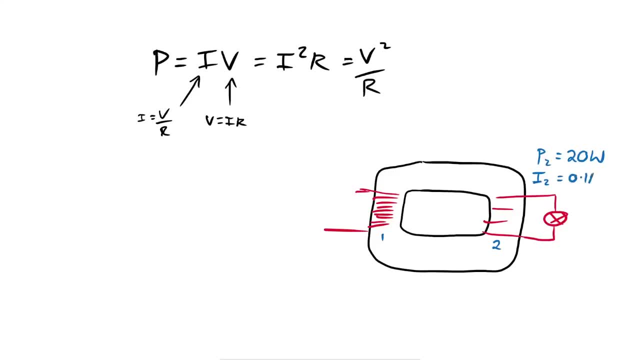 The current going through. it is 0.1 amps, So if that's the case, then we can of course use just this version of the power equation. We can say that V is equal to P divided by I, So that's 20 divided by I. 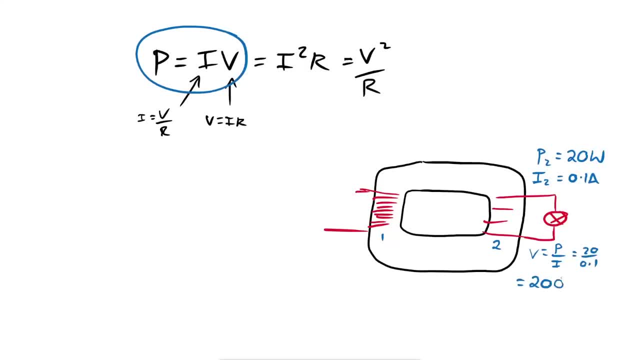 Divided by 0.1, that gives us 200 volts. That is a beastie bulb. So if that's the case, then you can just say that Here's our AC source. there, By the way, transformers are just for triple science. 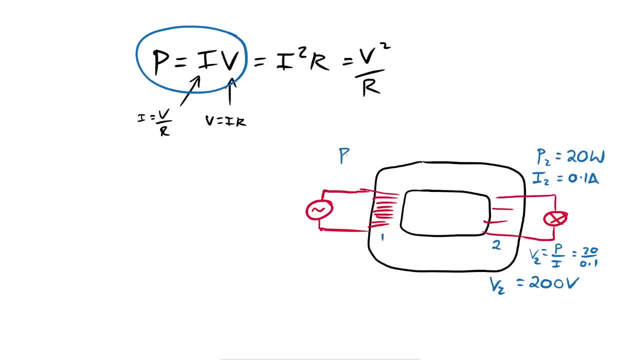 and A-level physics. If it's 100% efficient, well we can say: the power going in is equal to the power coming out. So we can say: power one is equal to 20 watts, and then we can go from there as well. 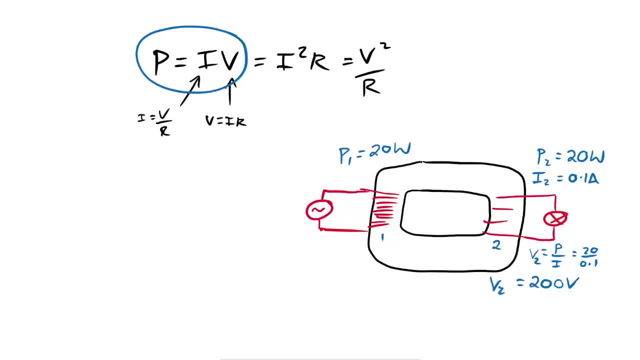 We can do our ratio of turns, et cetera, et cetera. Point is we're expected to use the power equation to find out V or I for a component. Now you remember I said V equals IR. I mean that is true for a component. 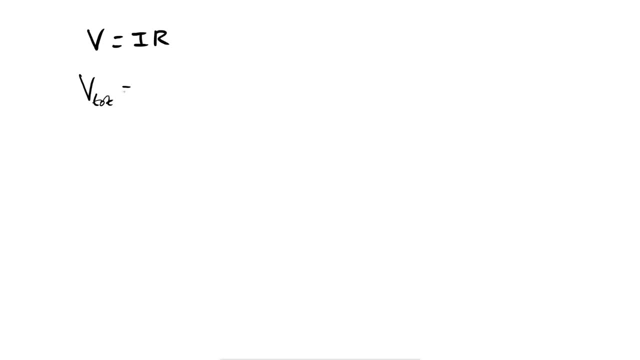 but it's also true for a whole circuit. So actually it's useful remembering that V total is equal to I total times R total for a whole circuit, Or like a branch or something like. that Point is you can use Ohm's law. 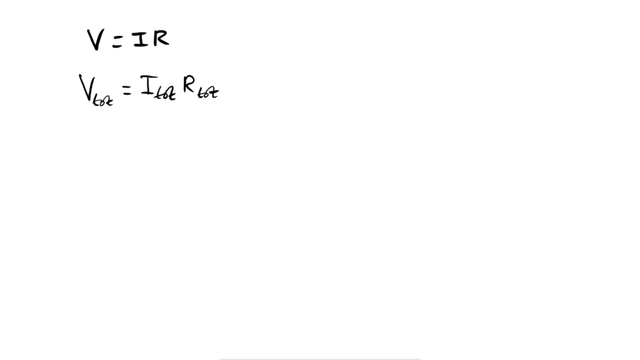 for a certain aspect of a circuit, not just an individual component. So if I have two resistors in series- these are 50 ohms and 150 ohms, let's say I have a battery that's 12 volts- then what can I find out about this? 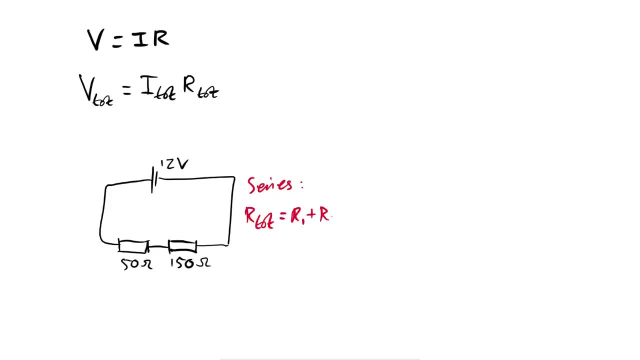 I can say that for series, total resistance is just equal to R one plus R two plus R three, whatever, however many resistances you have in series. So therefore, in this case it's going to be 50 plus 150, that's 200 ohms. 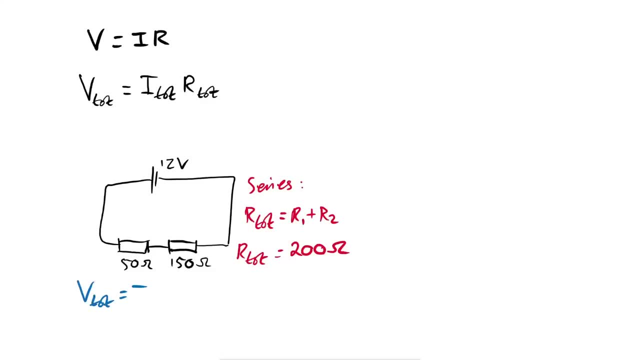 Therefore I can say that V tot is equal to I tot times by R tot. therefore, this total current is equal to the total voltage divided by the total resistance. So it's going to be 12 divided by 200.. That's going to give me 0.06 amps. 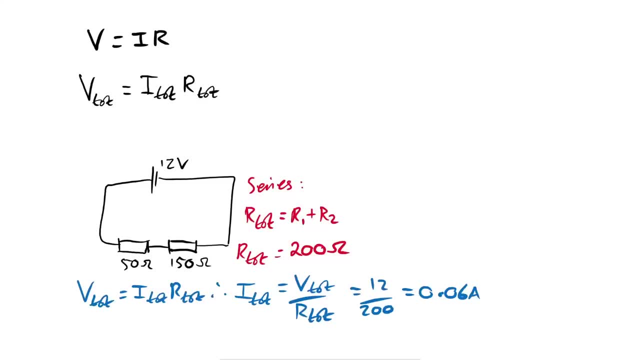 So if you're stuck looking at an individual component, if you don't have two things out of V, I and R for a component, look at the whole circuit, See if you can find out the total resistance. Little bit trickier when it comes to parallel circuits. 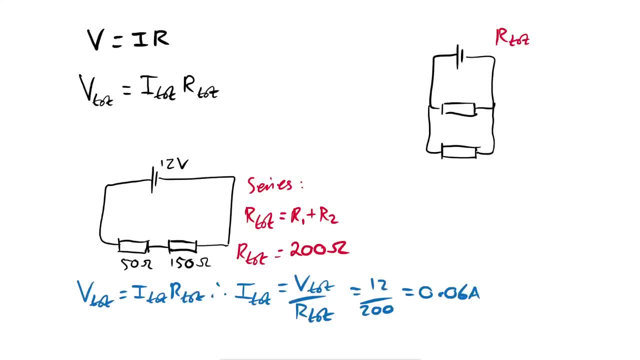 How do we find out the total resistance in this case? We have an equation for it. Let's derive it real quick, shall we? So let's say that we've got the total resistance of the current that's going through the two branches added up together. 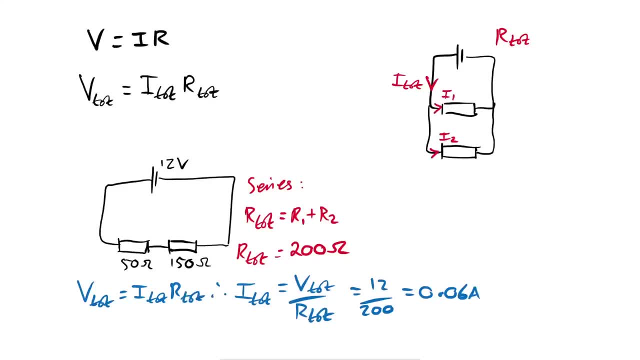 So we can say I tot is equal to I one plus I two. Of course we know that from Ohm's law I is equal to V over R, So we can just replace this with V tot over R. tot is equal to V one over R one, plus V tot over R two. 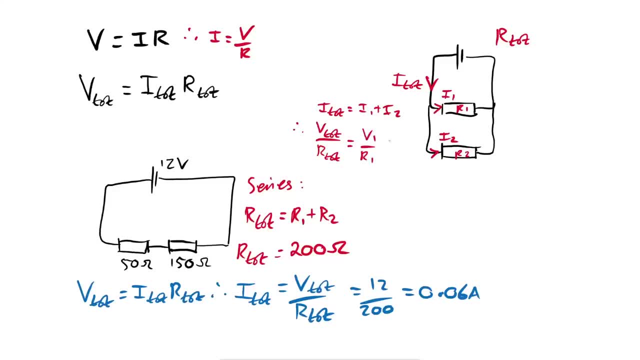 So that's going to give us the total resistance of the current that's going through the two branches. That's V two over R two. All I've done is replaced my currents with V over Rs for the individual resistors and the whole circuit. 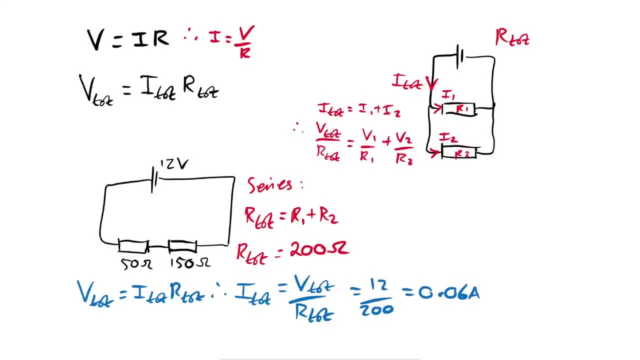 What do we know is true for voltages in a parallel circuit? We know they are the same. So actually, let's say the total voltage is six, It's going to be six for that, six for that. So actually they all cancel out. 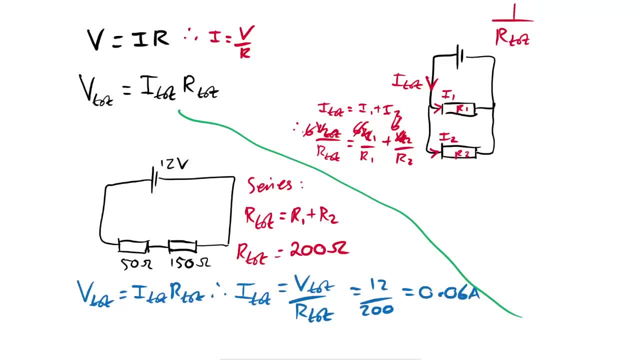 So therefore our equation for total resistance is one over R. total is equal to one over R one plus one over R two, et cetera. We add however many resistors we have in parallel. People get a little bit confused with this one. 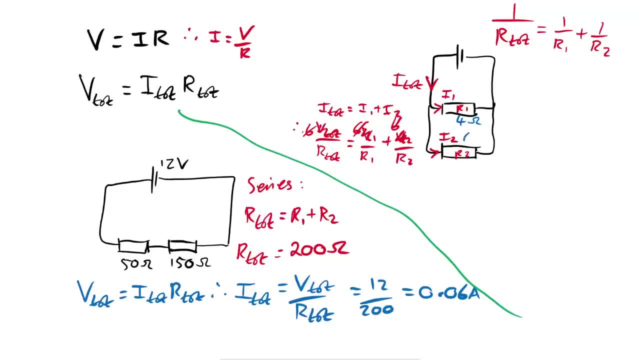 so let's have a go with some numbers. Let's say that this is four Ohms and this is six Ohms. Therefore, one over R, total is going to be equal to one over four plus one over six. What do we do with that? 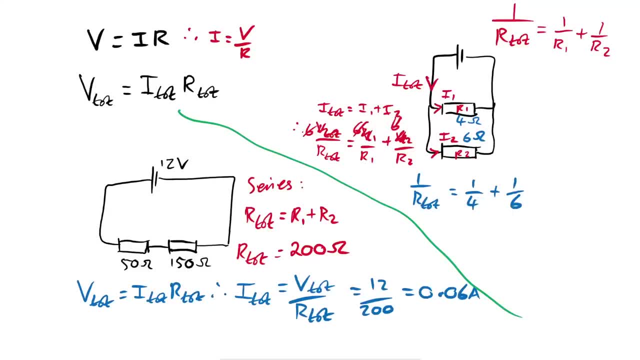 Well, let's find a common denominator, shall we About four and six? so let's go for 12.. So this is equal to three 12ths plus two 12ths plus two 12ths, and so that gives us five 12ths. 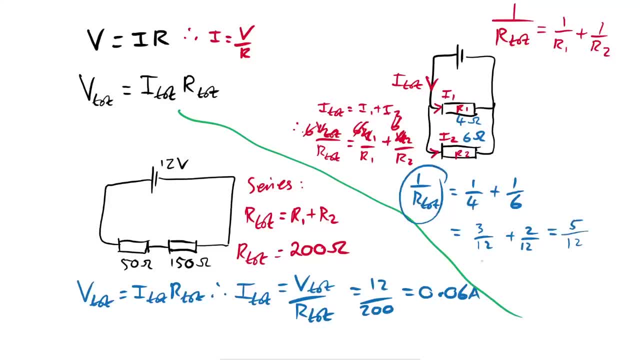 That's not our answer, though, because that's one over that, So therefore, all we have to do is flip it on its head. So R total is just reciprocal, is equal to 12 over five, and so that's 2.4 Ohms. 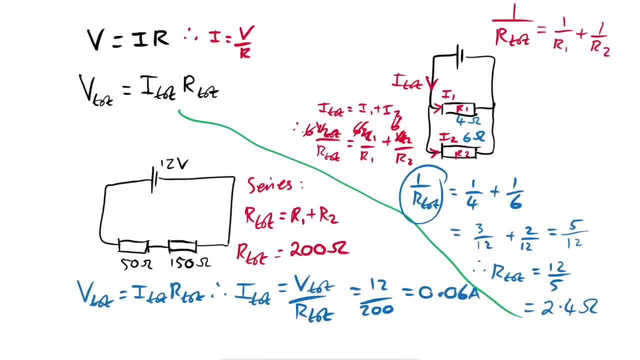 So that's how you find total resistance for a parallel circuit. You can then, of course, use that to find out total current or total voltage as well, depending on what the question is asking. So there we go. that's the basis of pretty much all electricity questions. 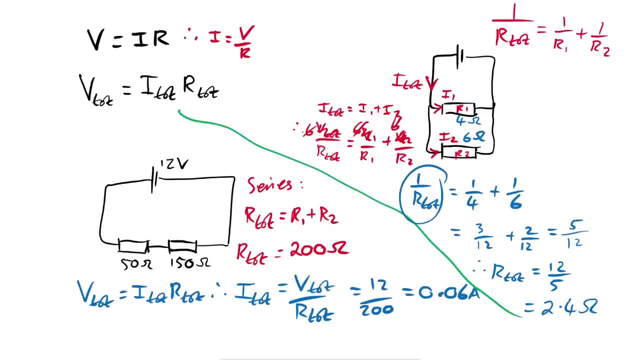 Even things like internal resistance and EMF. After all, that's just two resistors in series. It just so happens that one of the resistors is inside the battery, as it were. It's all about just keeping your head, just looking at. do you have two things for a component? 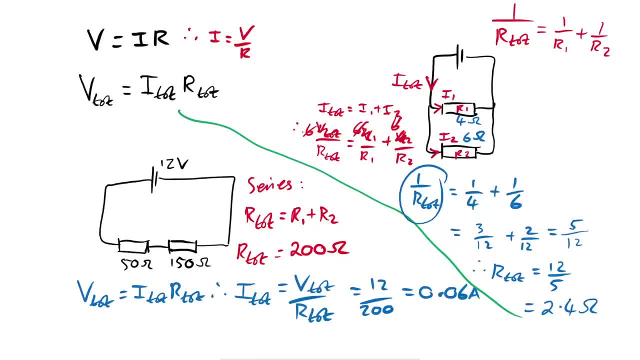 or the whole circuit. If so, then you can find out. third Chances are you're gonna use that third thing and then do a second calculation. That's usually how it goes, So I hope you found that helpful. If you did, please leave a like. 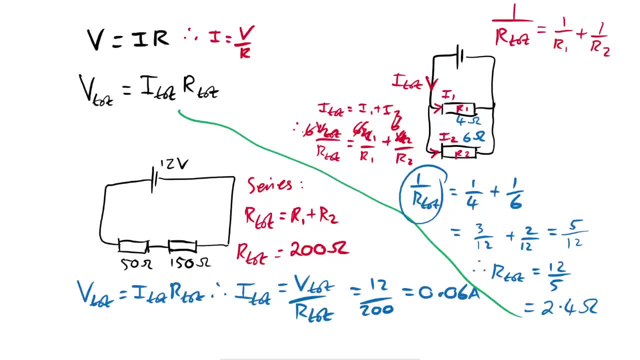 If you wanna have a look at my big electricity video, then click on the card. very helpful video. Thanks for watching. see you next time.